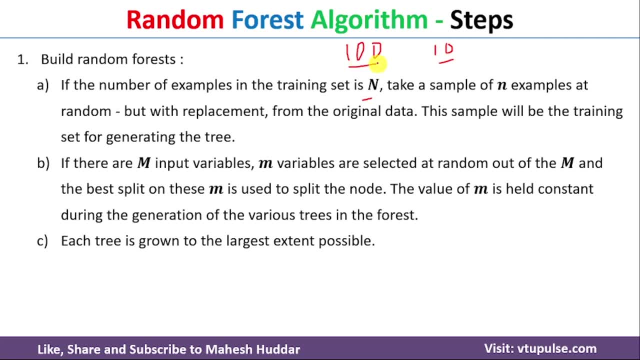 random forest. So this is the number of decision trees. This is the total number of examples given to us. Now what we do over here is we will select n number of examples. Let us say that we want to select 30 examples for each of those decision trees. So what we do here is: first, we will select 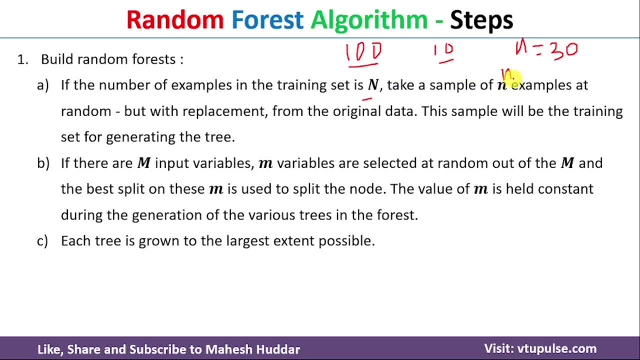 30 examples out of 100. So that will become, you can say that, n1. that will be the first training example for the first decision tree. Next, what we do is we will put this particular 30 examples again back into this particular total number of training examples Out of. 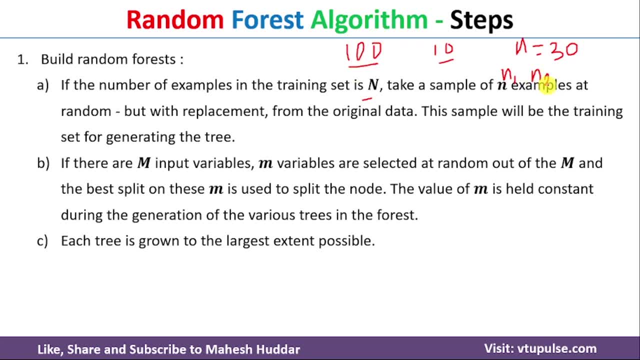 100, again we will select one more set randomly. that is 30 examples. Once you select one more set, we will put those examples again back into this training set and then we will select another 30 examples, and so on 10 times or 10 sets we will select here. So whenever we select some examples, 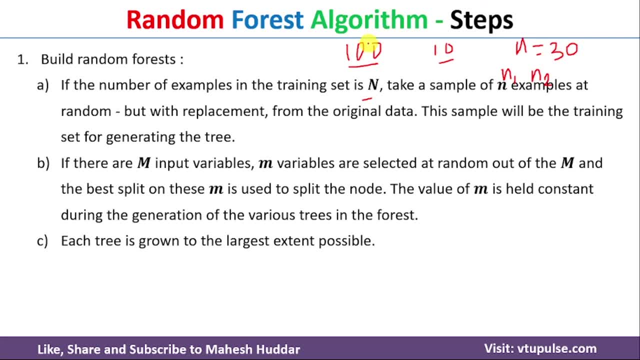 or a subset of examples, randomly. we will put them back into the training set over here. So once you do this part, I think the second step is to select the input variables. Let us assume that we have 10 input variables. While building each of those particular decision trees in the random forest. 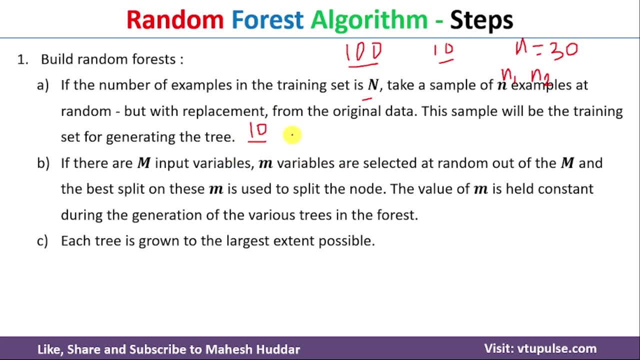 we need to select subset of these particular 10 variables. Let us say that I will select five variables. So what we do is, in the first step, we will select five variables randomly, and then we will put it back, and then again we will select five variables, and so on For each. 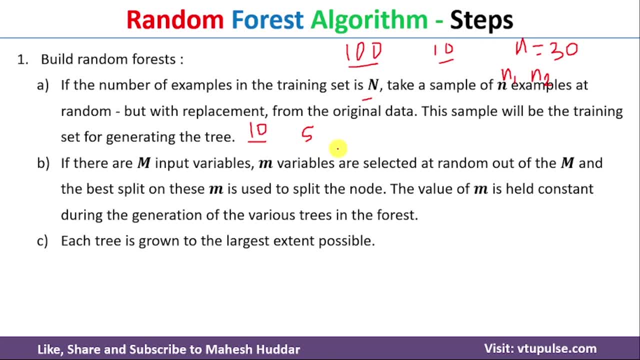 of those particular 10 different decision trees. we will select five features over here, because we are putting it again back over here. we will get a mixture of all those particular variables in this case. So once you get the training set for all 10 decision trees, 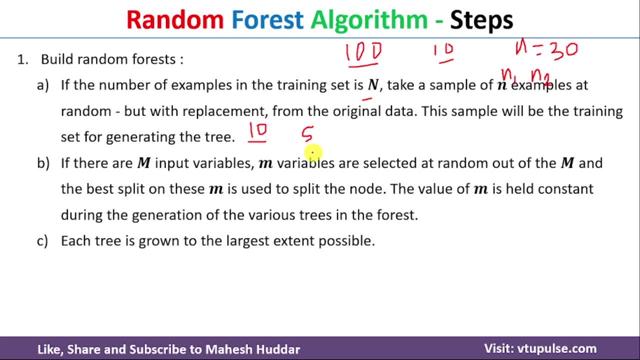 and the feature features, or you can say that the input variables. next, what we do is we will build the decision tree using the decision tree algorithm. So once you build the decision trees of random forest, whenever we get a new data point, we give that new data point as an input to that. 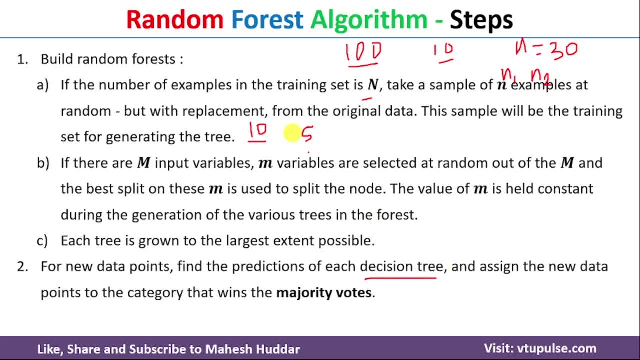 particular random forest, that is, each decision tree in the random forest. So in this case we have 10 number of decision trees in the random forest. each of those particular 10 decision trees will make 10 different predictions over here. now the question is how to assign the label to this. 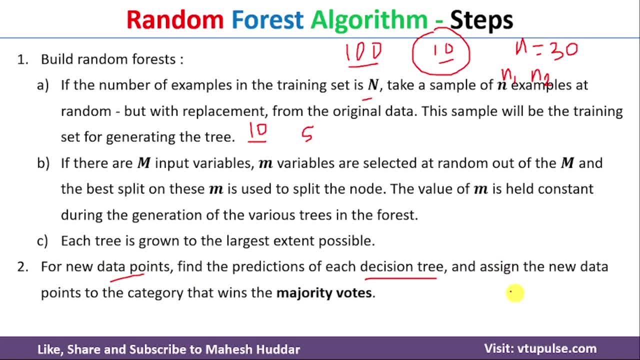 particular new data point. so what we do over here is, if it is a classification kind of problem, we will take majority of that particular 10 decision trees, the one which is having maximum votes. that will be selected as a label for this particular new example. if it is a regression kind, 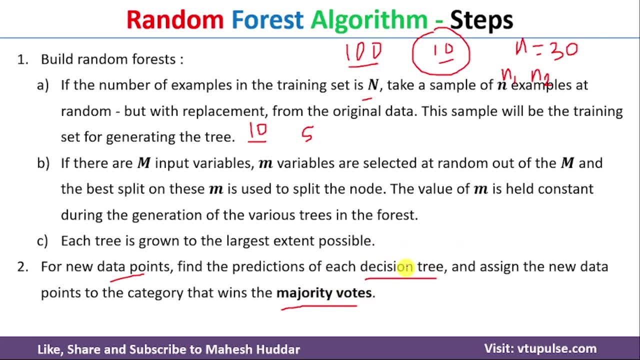 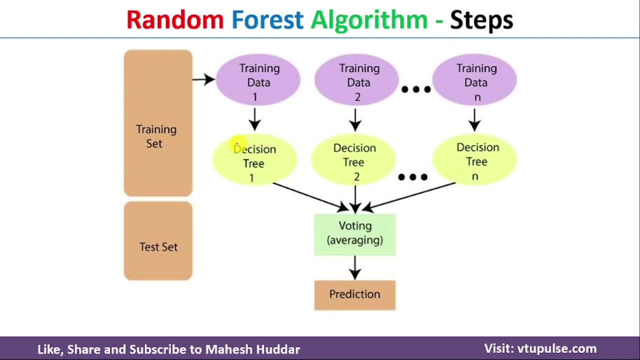 of problem, then we will take the average of 10 decision trees predictions. that will be considered as the final case over here. this is the diagrammatic representation of random forest algorithm. this is the training set. the training set is divided into multiple number of training datas. let us say the. 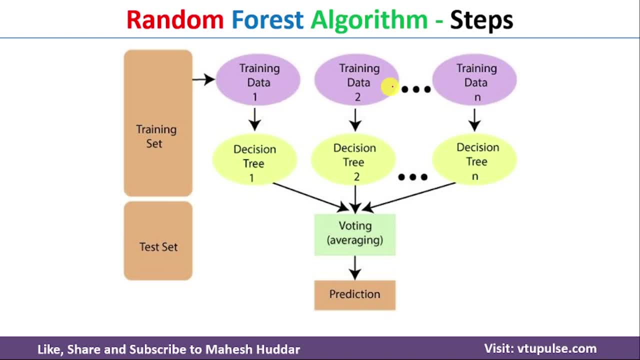 training data 1. training data 2. training data n: over here. with the help of this particular training data, we will train the decision trees. that is nothing, but we will build the decision trees and then we will give the new example to these decision trees. each of these particular decision trees will make the predictions and then 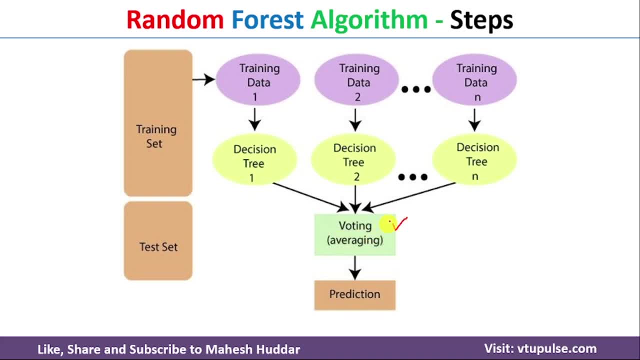 what we do here is we will take the majority for classification problems. if it is a regression, we will consider the average of those particular probabilities and then we will make the final prediction over here. so this is how the random forest algorithm works. now, coming back to an 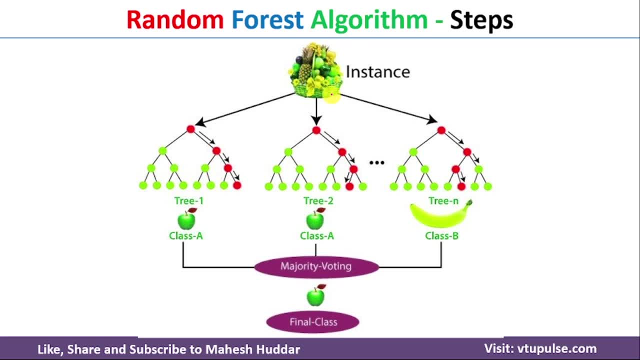 example of random forest algorithm. let us assume that we want to classify the fruits over here. there were a lot of fruits are there. we want to classify those particular fruits. so what we do initially is we will divide this particular fruits into a different training datas. let us say that there were 100 fruits are given to us. we will divide those. 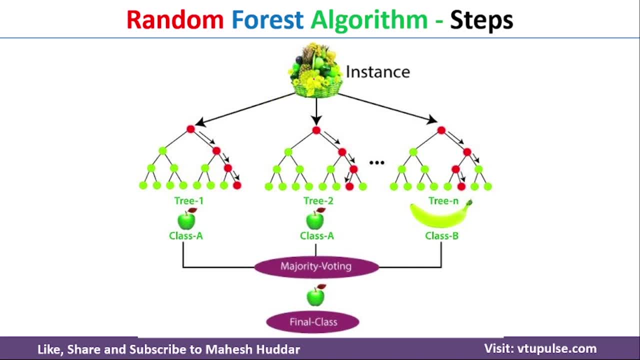 particular thing into. let us say that 30, 30, 30. so, using those particular three data points, what we do is we will build the decision trees. let us say that this is the first decision tree, second decision tree and third decision tree. now, once you build this particular decision tree, we will. 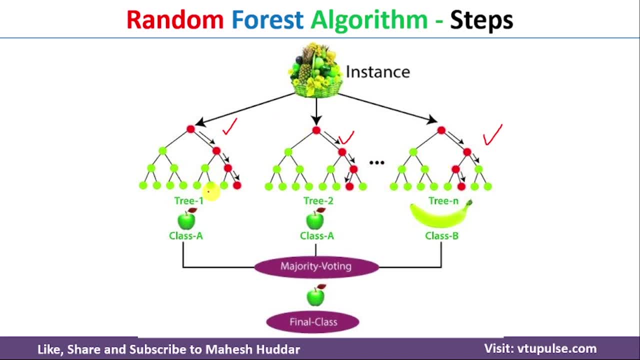 give the new example as an input to these particular decision trees, so that the new example will be classified by this first tree as apple in this case. second one as apple again. the third one is classified as banana in this case now, because it's a classification problem. 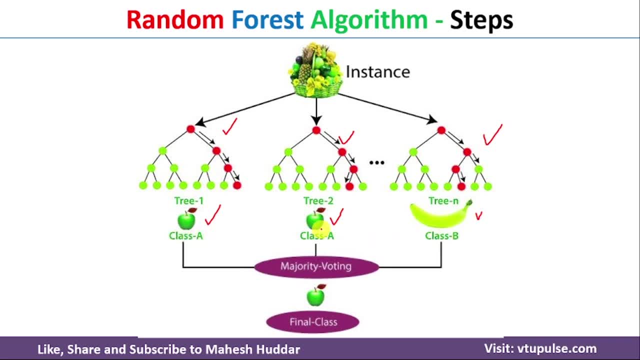 we need to take the majority voting here. in this case, the apple is coming two times and banana one time. hence, the new example will be classified as apple, because apple is having a majority in this case. now this is how we can classify the new example into one of the classes, using random forest. 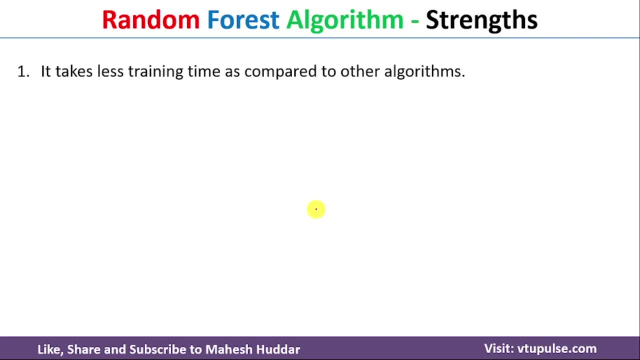 algorithm. now coming back to the strengths of random forest algorithm, it takes less training time as compared to other algorithms. actually, when you compare the training time of random forest algorithm with other ensemble learning techniques, like boosting algorithm, it is comparatively less over here, as well as it is comparatively less compared to other 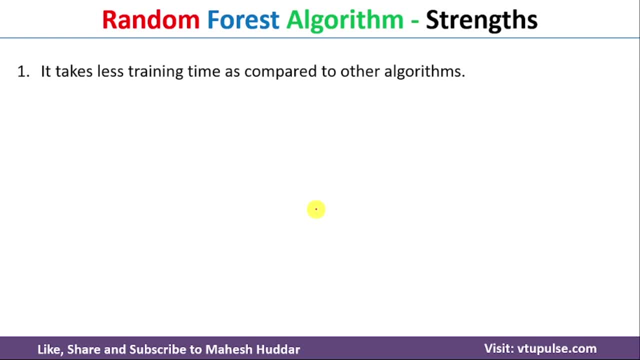 traditional machine learning algorithms like svm and so on. it predicts output with high accuracy. even for the large data set it works efficiently. that's a very interesting strength of random forest algorithm. it can also maintain the accuracy when we have a large portion of the data, where the missing data 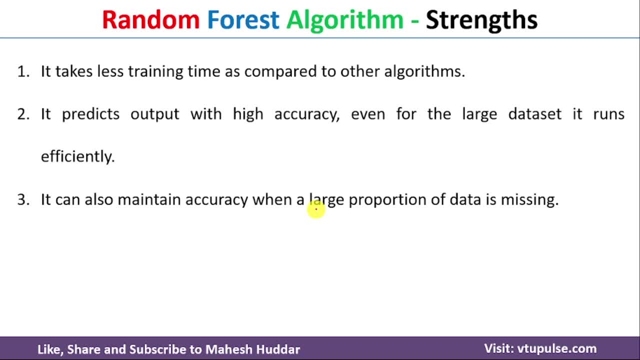 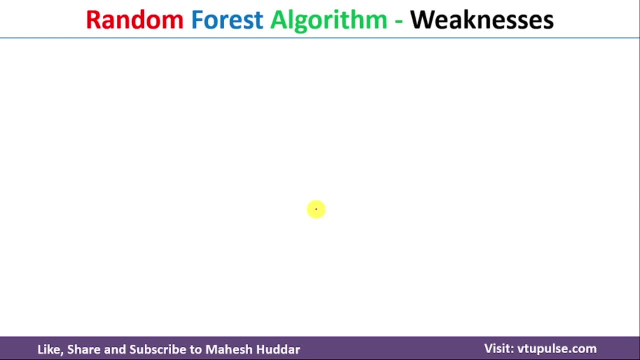 is there, or outliers are there, or some noisy data is there? still? the random forest algorithm gives a better accuracy over here. coming back to the last part of this discussion, that is, the weaknesses of random forest algorithm. the first weakness of random forest algorithm is whenever we have a classification problem, the random forest algorithm works perfectly fine. 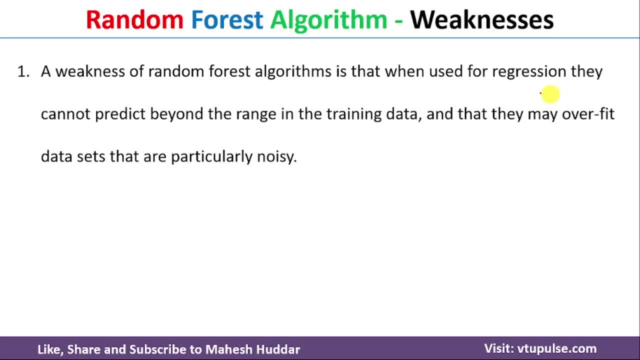 there will not be any issues. but when you have a regression kind of problem, the regression kind of problem actually gives you the numerical data as a result, in this case. but this will not work beyond the training data. for example, your training data contains the numerical column or the target. 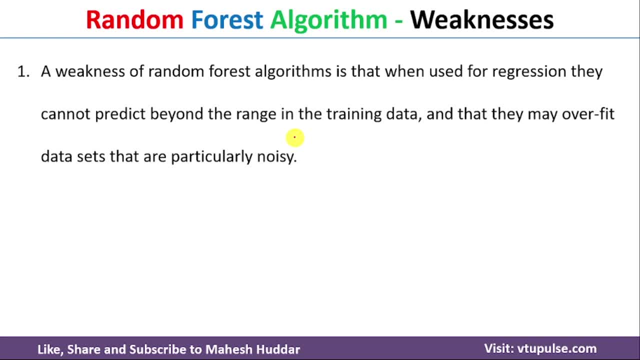 column in the range of 1 to 100, it will work only for 1 to 100. if you have a new data point which is beyond 100 or below 1, it will not work over there. that is the one disadvantage, or the weakness, of random forest algorithm. sometimes let us say that the data containing noisy data, 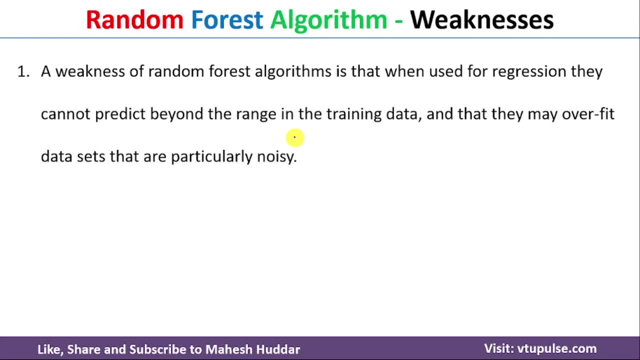 there is a possibility- it is not always, but there is a possibility- that the random forest may go into overfitting. that's the one more issue. when we build a random forest algorithm, because we are going to build multiple number of decision trees, it will take a lot of space on.